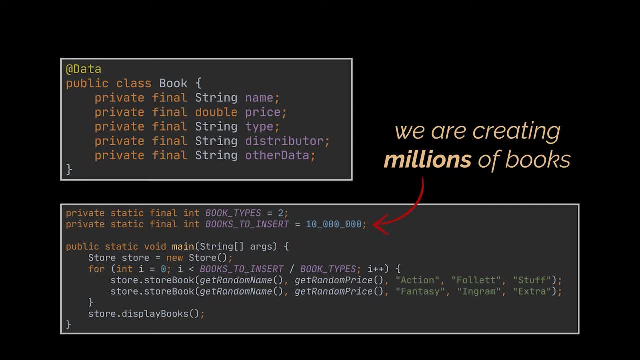 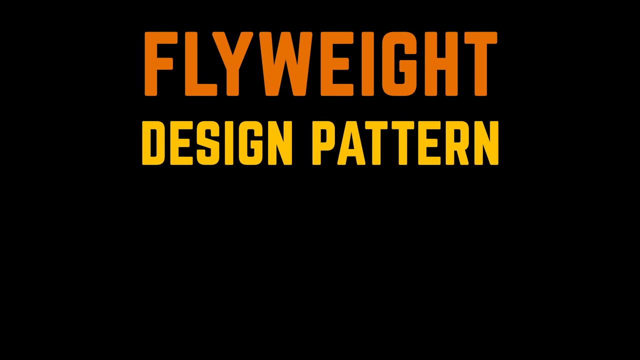 Hence we were trying to render millions of big objects, and these created objects no longer fitted in the remaining RAM of your manager's laptop, So the program crashed. A solution to the problem we are facing could be to apply and implement the flyweight design pattern. 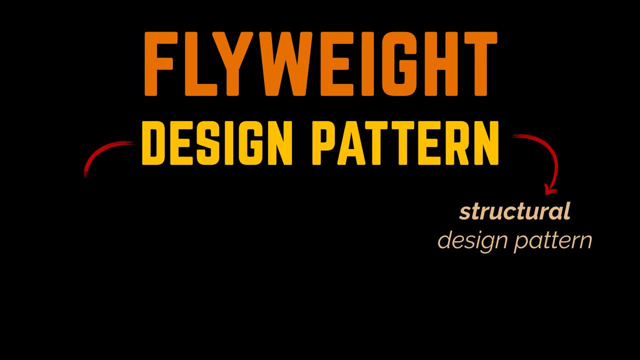 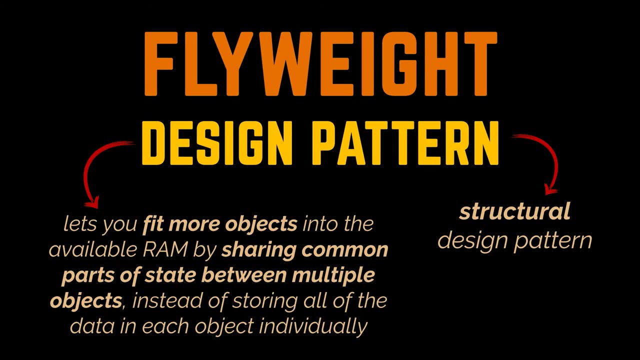 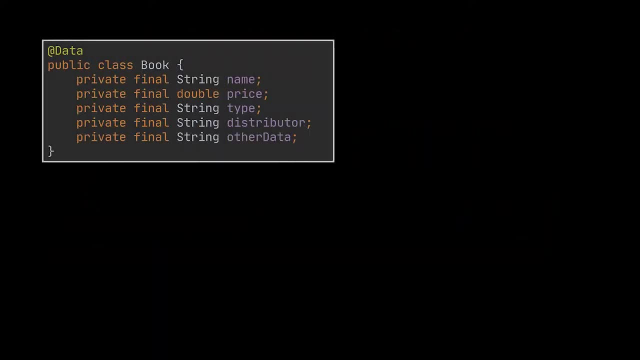 This pattern is a structural design pattern that lets you fit more objects into the available amount of RAM by sharing common parts of state between multiple objects, instead of storing all of the data in each object individually. To break this down, let's apply the flyweight pattern on this example. To do that, we need to 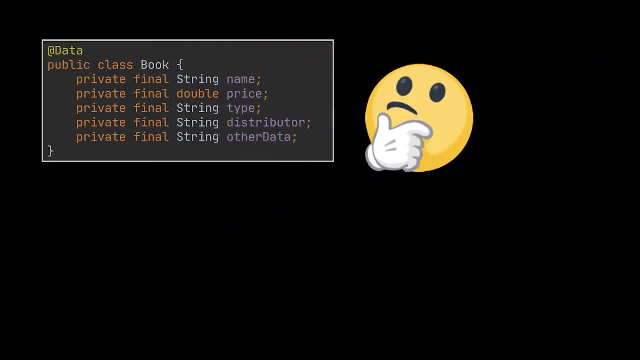 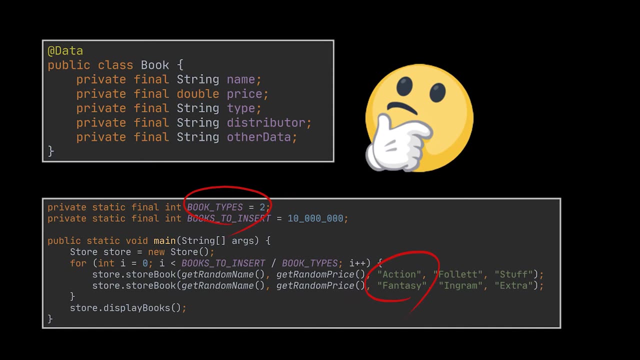 take a closer look at our book class and try to identify, if they exist, common attributes shared across our book objects. On closer inspection, you can notice that the type attribute takes only two values- action and fantasy- And whenever the type takes a particular value, both the distributor and 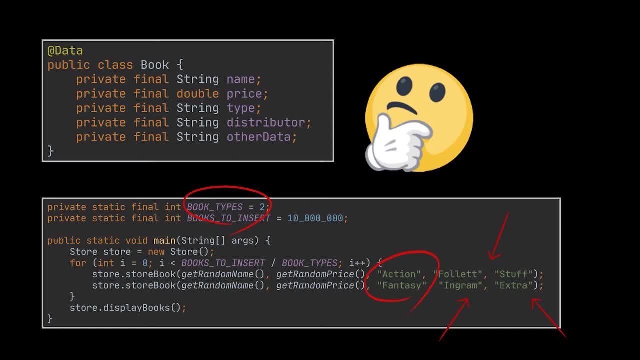 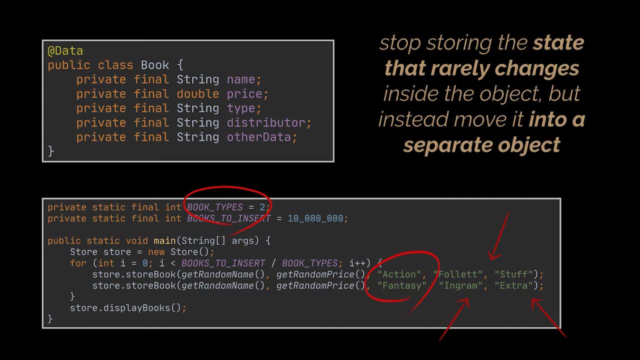 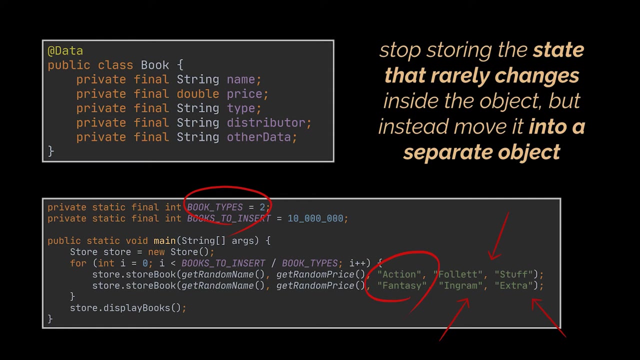 data attributes will follow on the same values, So the distributor of all of our action books is the same one, for example. In this case, the flyweight pattern suggests that you stop storing the state that rarely changes inside the original object, but instead move it into. 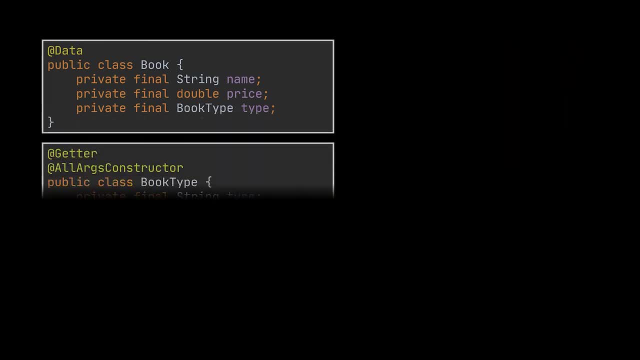 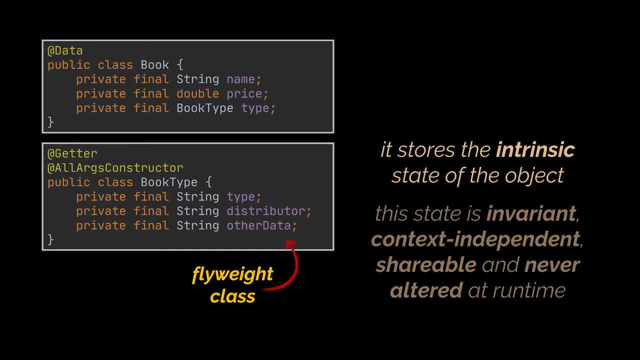 a separate object. Let's move our three repeating attributes to a new class and name it book type. This class is what we call the flyweight class and it stores the intrinsic state of the object. This state is invariant, context independent. 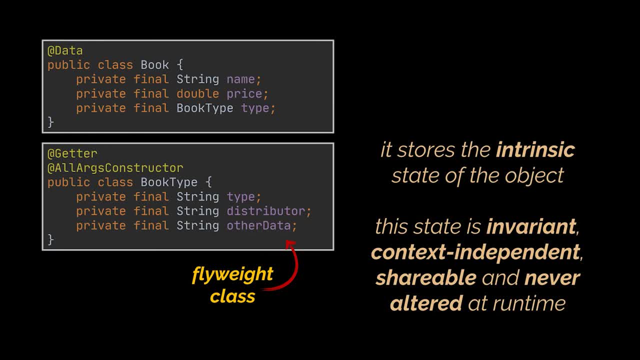 shareable and never altered at runtime. And since the same flyweight object will be used by many books in this example, we have to make sure that its state can't be modified. So the book type class should initialize its state just once via constructor parameters. It shouldn't expose any 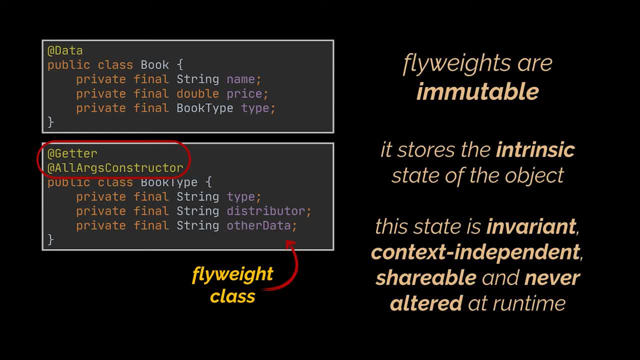 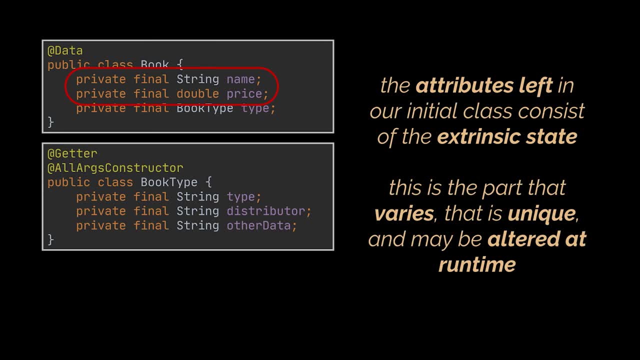 setters or public fields to other objects. The attributes we left in our initial book class consist of the extrinsic state of the object. This is the part of the object that varies between one another, that is unique and may be altered at runtime internally by our application. All that is left to do now is define these. 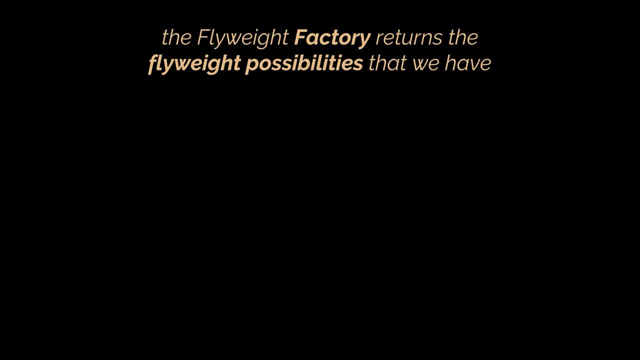 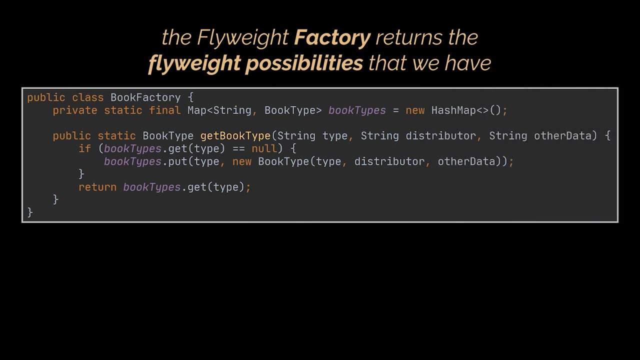 types, the flyweight possibilities that we have, And this is done using a flyweight factory. This class usually consists of a map to cache the values of our flyweights, and whenever a book type object, let's say, is requested, a new flyweight object is created for it and stored inside this. 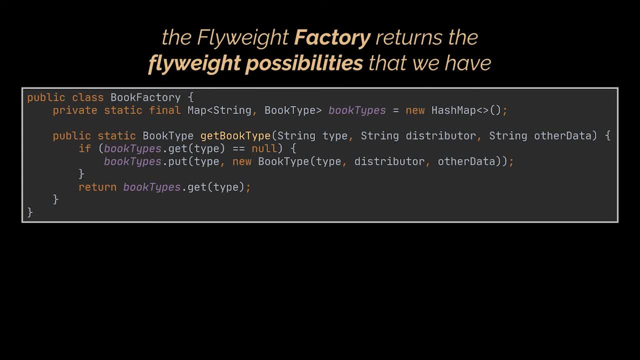 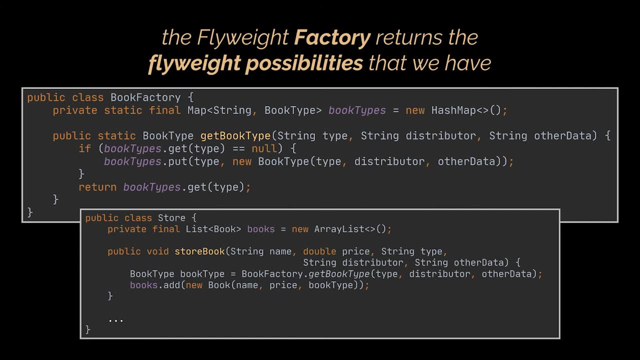 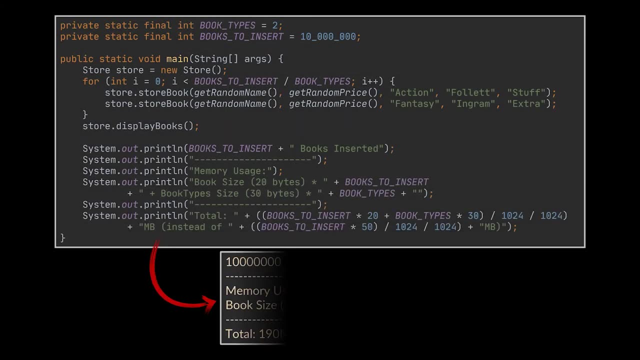 map, making it reusable by all the objects that need it Now in our store class. instead of just creating and storing the books we created, we first fetch the corresponding flyweight object for that book and then proceed by storing it. By doing that, and as you can see, if we consider 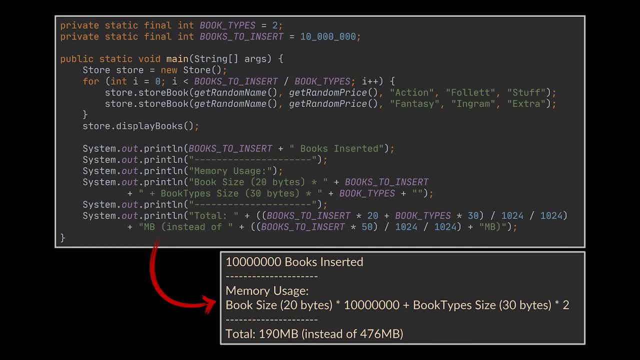 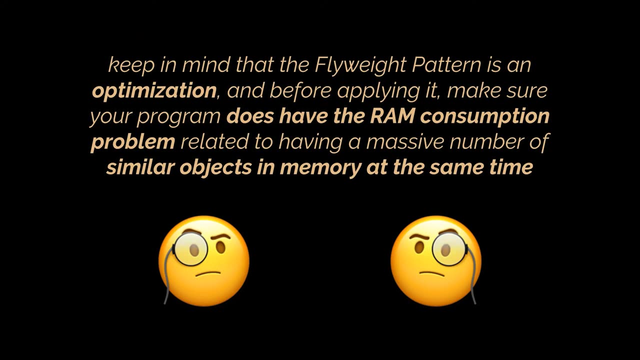 that each attribute stored in our book object has a size of 10 bytes, we managed to reduce our memory consumption by more than half. Okay, but this does not mean that we should split every object's state we have into intrinsic and extrinsic. Just keep in mind that the flyweight pattern is 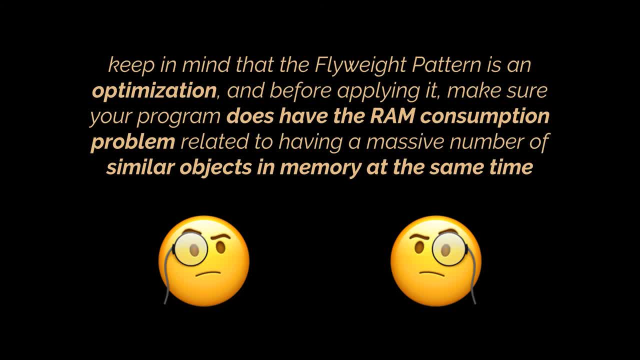 merely an optimization. Before applying it, make sure your program does have the RAM consumption problem related to having a massive number of similar objects in memory at the same time, same time. Okay, with that said, let's go ahead now and take a look at the structure or class. 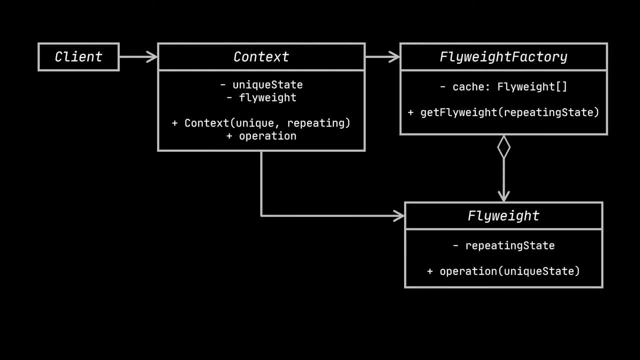 diagram of the flyweight design pattern while trying to relate it to the books example we just implemented. The first thing you will notice is, of course, the flyweight class, which was the book type class in our example. This class contains a portion of the original object's state that can. 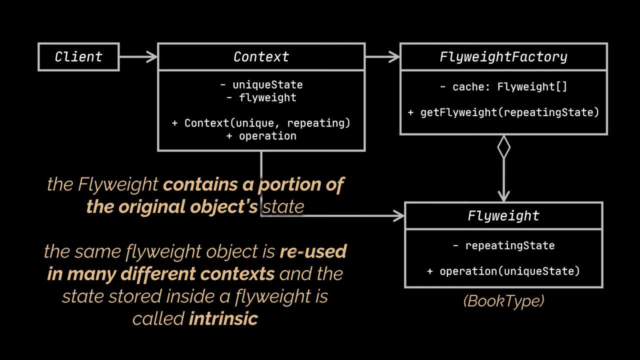 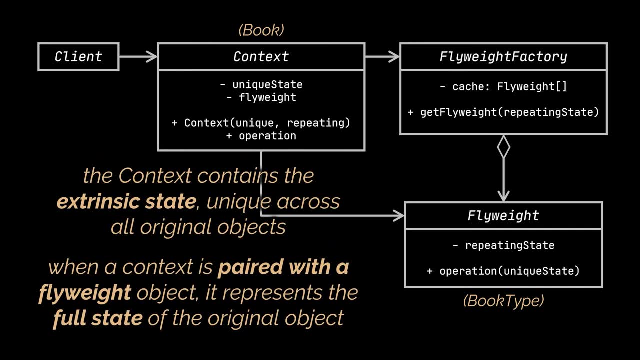 be shared between multiple objects. The same flyweight object is reused in many different contexts and the state stored inside a flyweight is called intrinsic. Next is the context class, which was the book class in our example. This class contains the extrinsic state unique across. 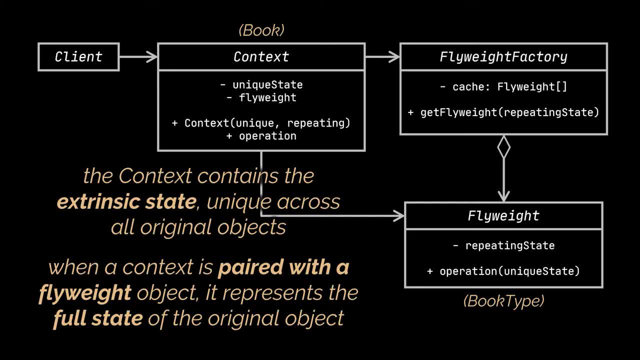 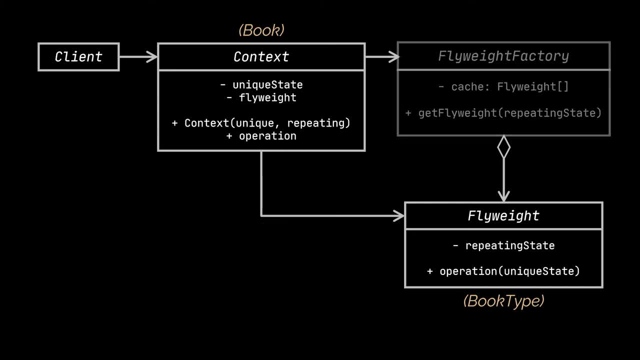 all original objects. When a context is paired with one of the flyweight objects, it represents the full state of the original object. Now, to create the flyweights, what we need is the flyweight factory. This class manages a pool of existing flyweights. 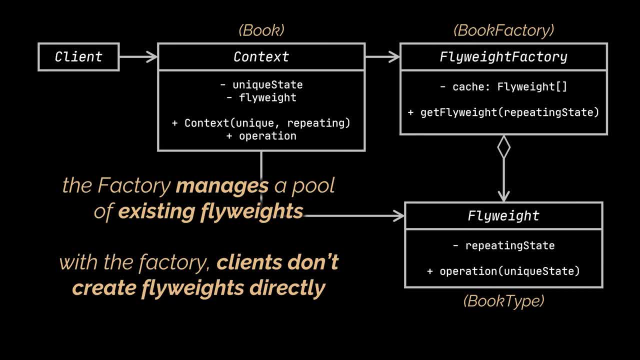 With the factory. clients don't create flyweights directly. Instead, they call the factory, which looks over previously created flyweights and either returns an existing one that matches the provided search criteria or creates a new one if nothing is found. Finally, we have the client. 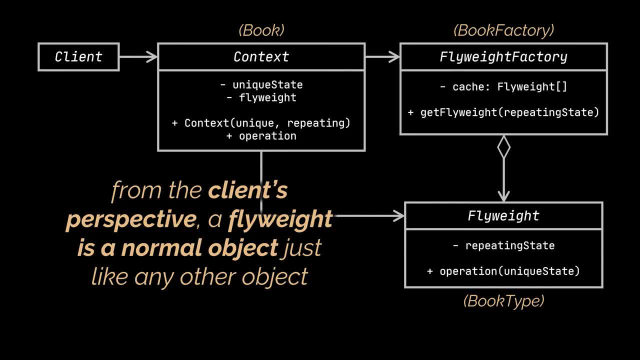 From the client's perspective, a flyweight is a normal object, just like any other object To them. it can be configured at runtime, as it is part of the context. So, to sum everything up, a flyweight refers to an object that minimizes memory usage by sharing.